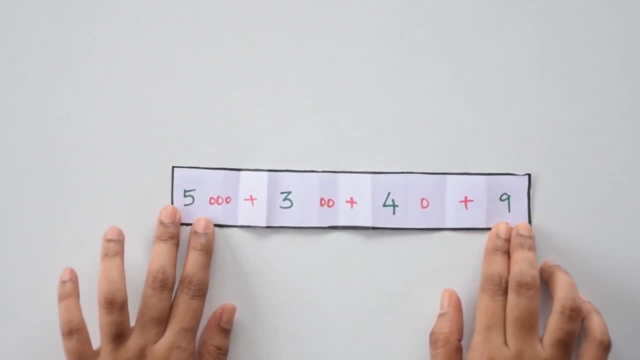 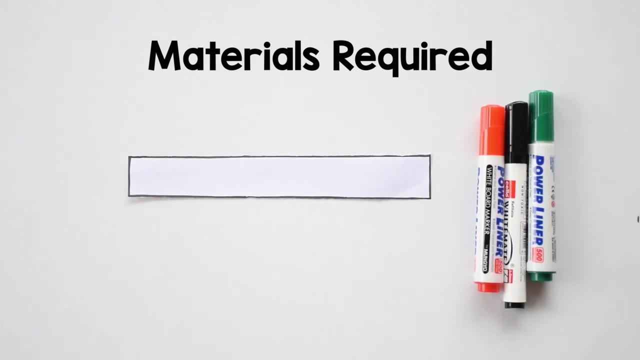 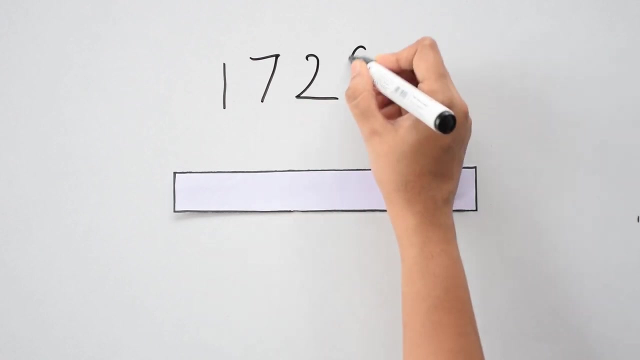 this a very simple and effective way of learning place values. Let's look at how it's done For this activity. all we need is a paper strip and a pen or pencil. Here we have used sketch pens. for better visibility, Let's take the number 1729.. Let's make the place value. 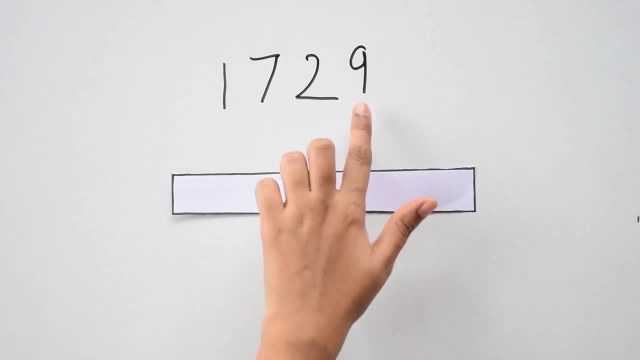 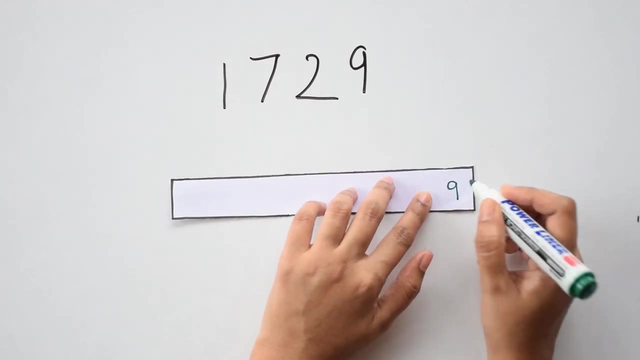 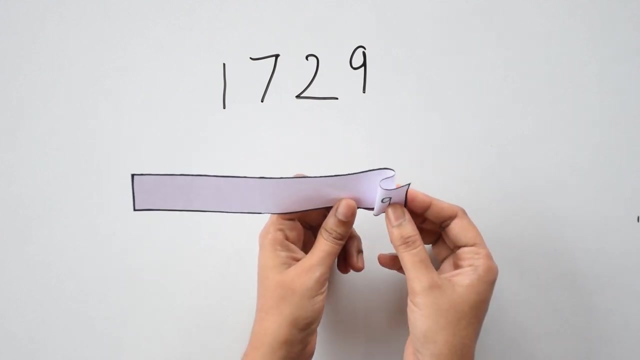 paper strip with this: First we'll take the number which is in the ones place, which is 9 here, and we'll write this in the right most corner. Next we'll take the paper and push the left side into the right such that a small flap. 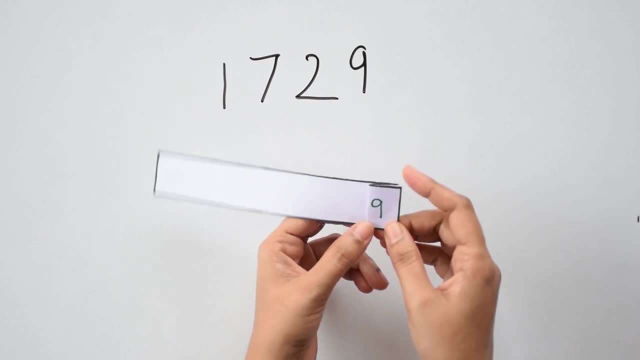 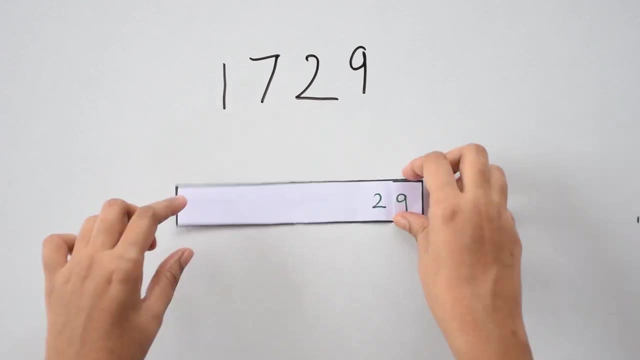 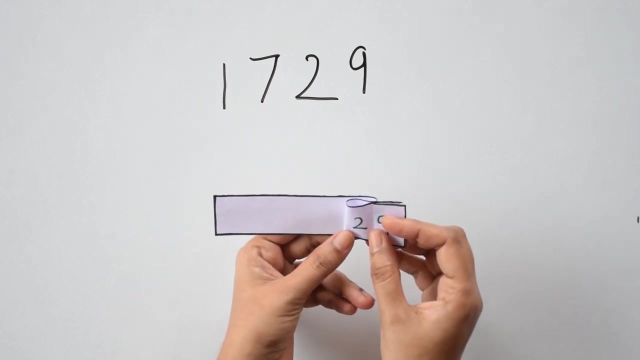 is created like this and the number 9 is visible. Let's take the next number here, which is 2.. We'll write it down here. Now. we'll repeat the same thing which we did, That is, push the left side into the right such that a small flap is created. 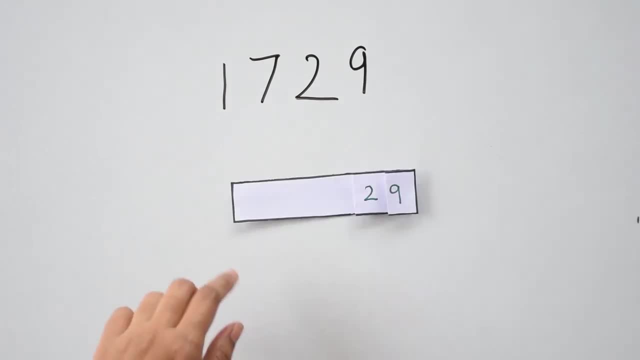 And the number 2 is visible. Let's take the next number here, which is 7.. We'll write it down and repeat the same activity, making sure that this number 7 is visible And we have a flap here. The last number is 1.. Let's write that down here. Now we have the number 1729.. 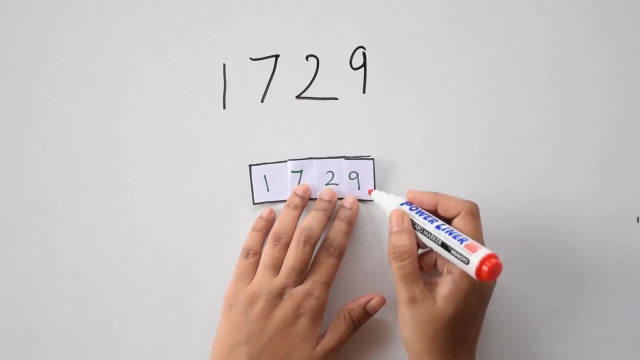 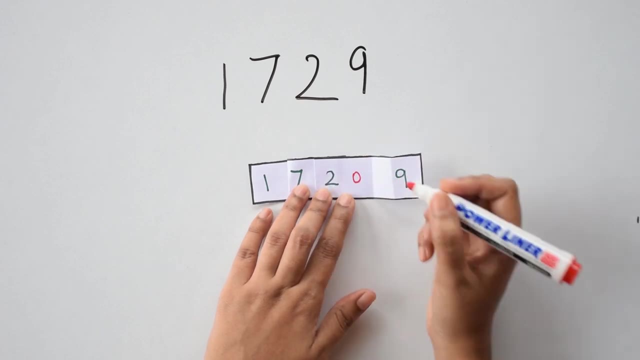 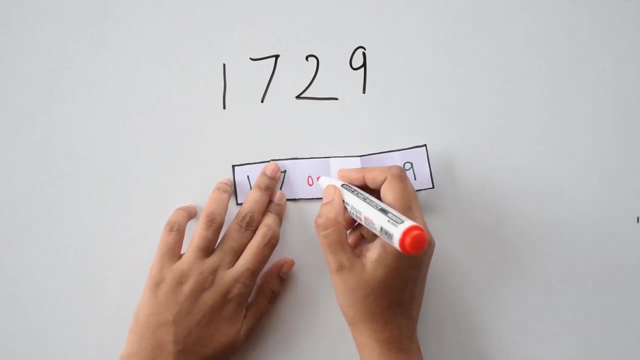 Let's look at the place values. 9 is in the ones place, so it can be as such. 2 is in the tens place, so we add a 0.. 7 is in the hundreds place, so we add two 0s. 1 is in the thousands. 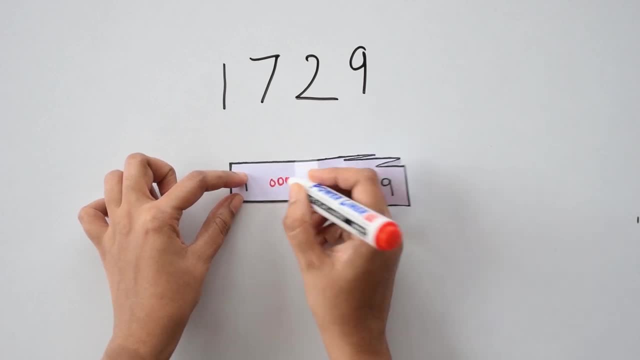 place. so we add three 0s. Now our paper strip is ready. Similarly, can you make a place value strip for the number 1988 and tell us the place value of the paper strip? Let's look at the place value of 9.. We would love to see your work. Please send it to the number. 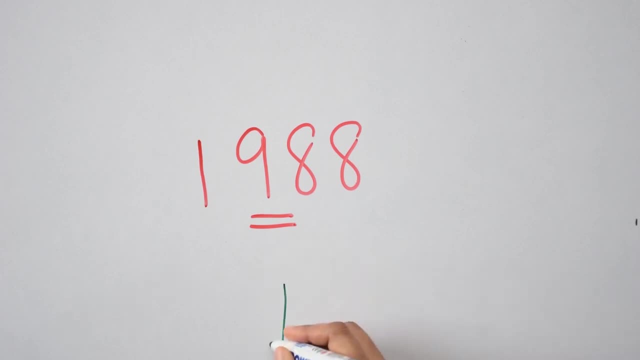 given below through WhatsApp or mail it to the mail id given below. Thank you for watching and stay tuned for more interesting videos.